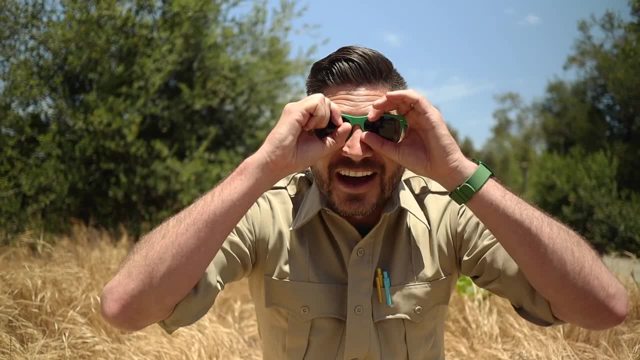 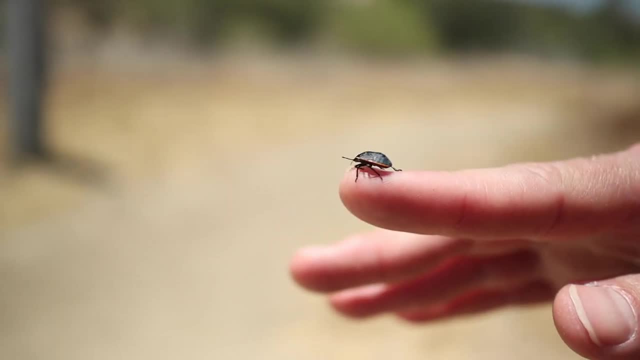 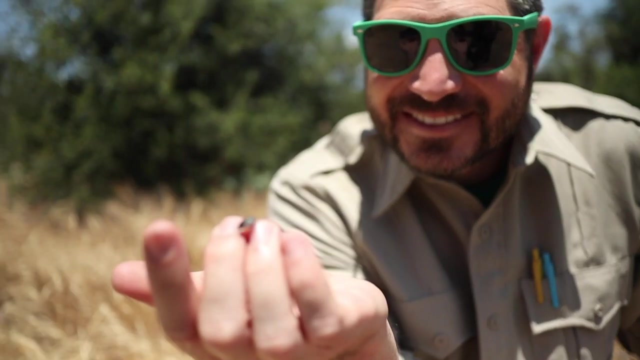 When we use our observation skills, hawk eyes- it's called using our sense of sight. When we look at something like this beetle here, what we're actually looking at is reflected light. Light bounces off an object and into our eyes. Our eyes then send the information to our brain and our brain. 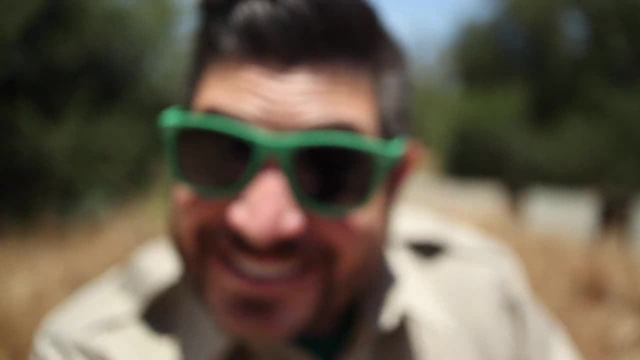 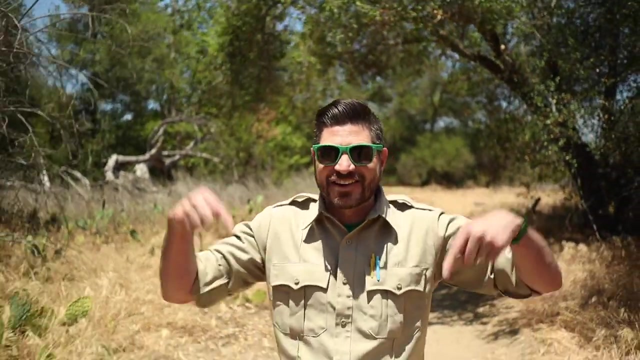 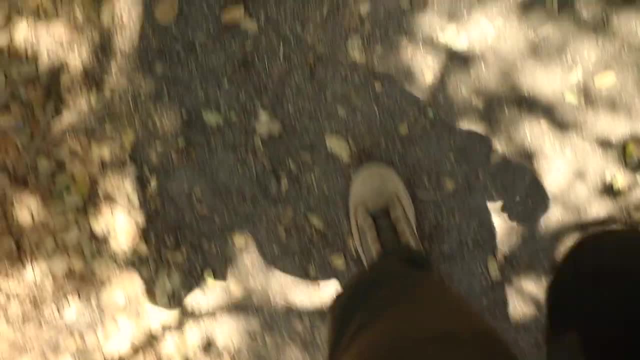 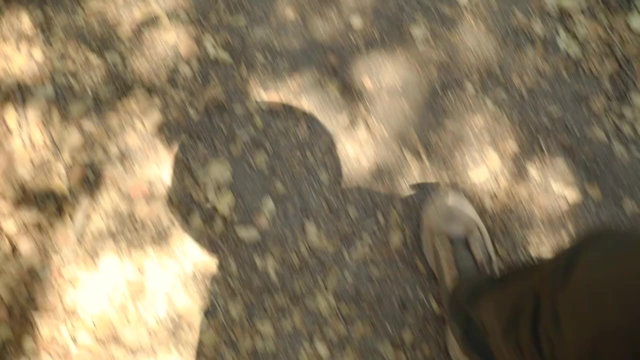 Here. let me show you just what I'm talking about. Here's what your hike is going to look like if you're only looking down at your feet. Pretty boring, And this is what you might see when you're out on a nature hike. 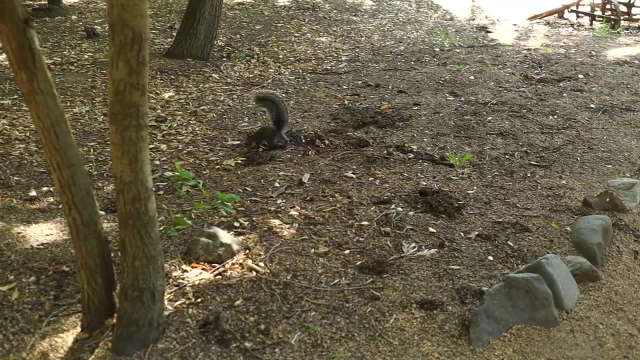 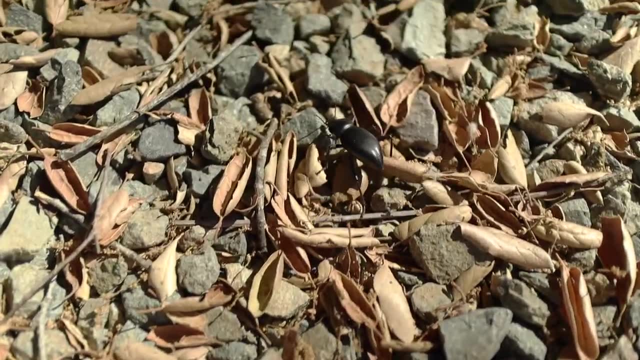 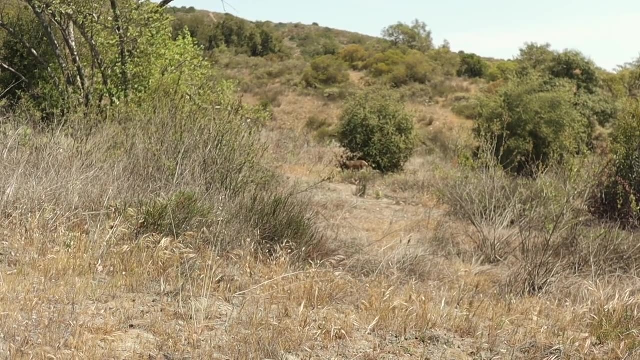 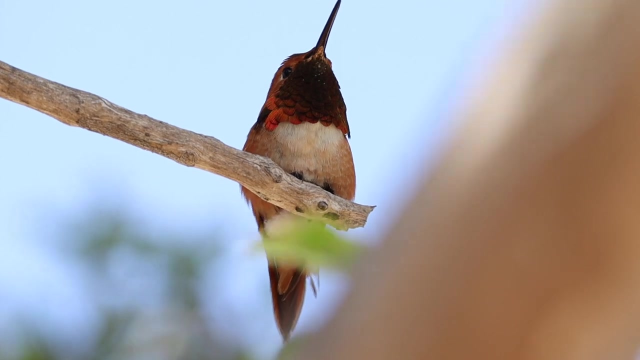 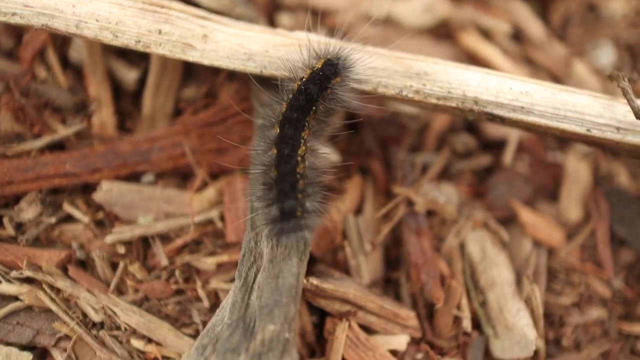 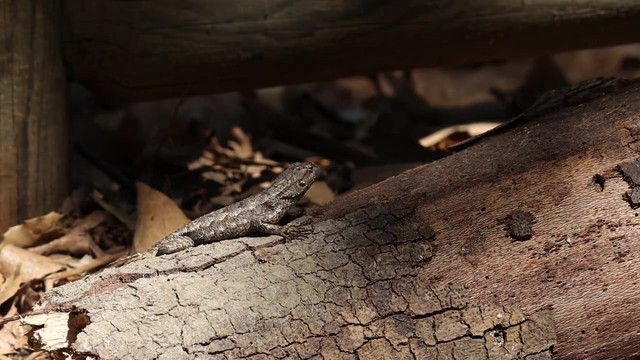 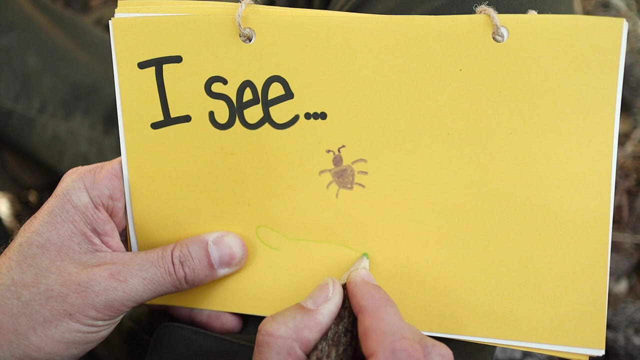 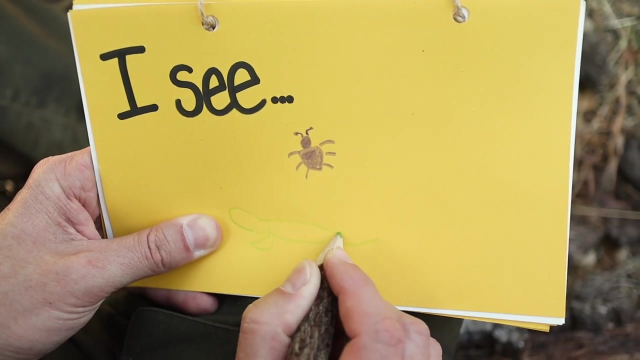 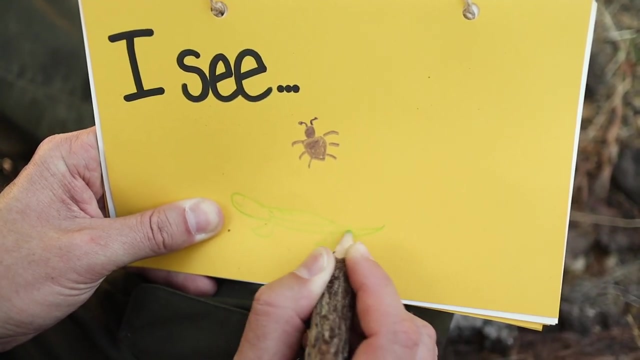 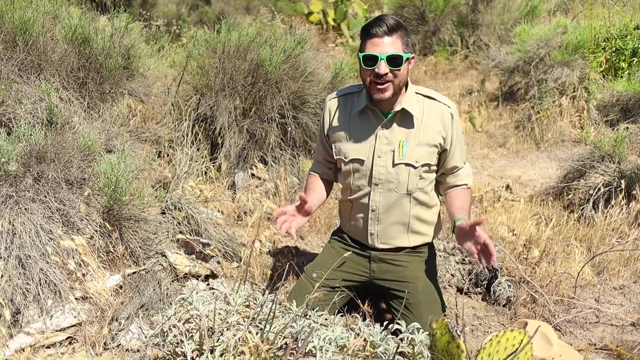 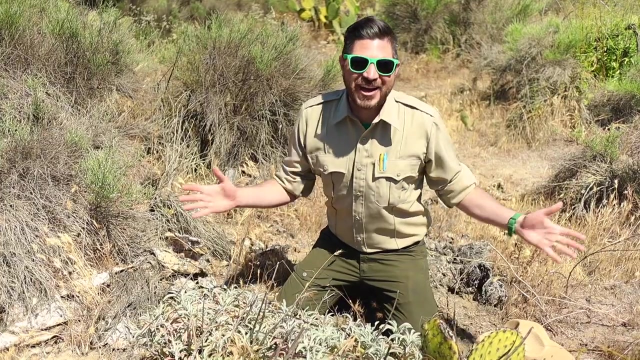 Let's see if you open up your hawk eyes. Here's what you might see when you're out on a nature hike. When we use our bare nose for observation, we are using our sense of smell. Just like your skin has touch receptors, our nose has smell receptors. 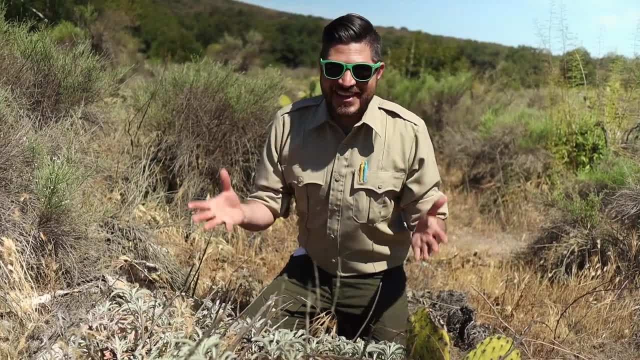 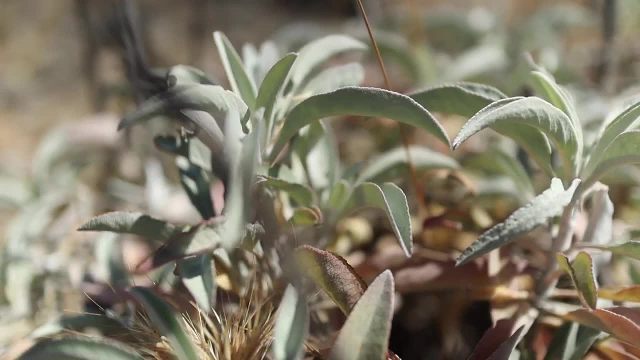 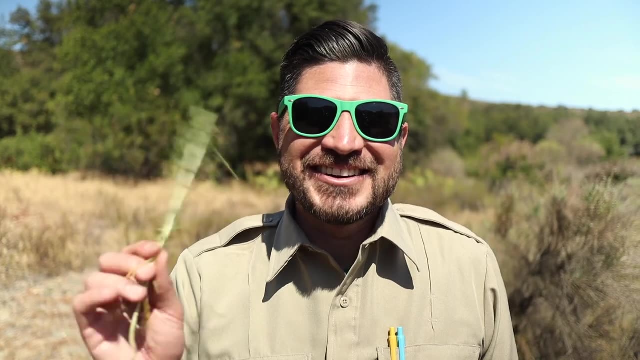 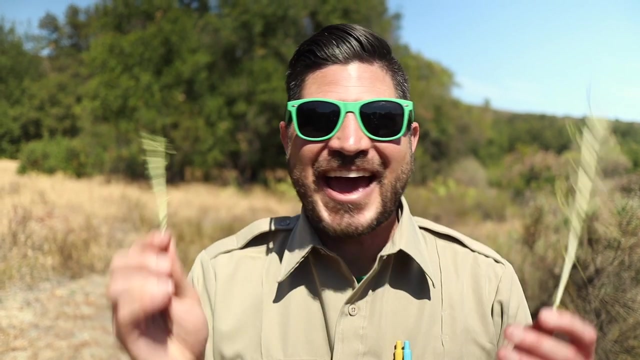 These smell receptors can tell us a lot about the things that we sniff. Some things smell really good, like this white sage, And other things can smell really stinky. Here's another plant that's worth sniffing. This is California sage, and it smells so good it's got the nickname Cowboy Cologne. 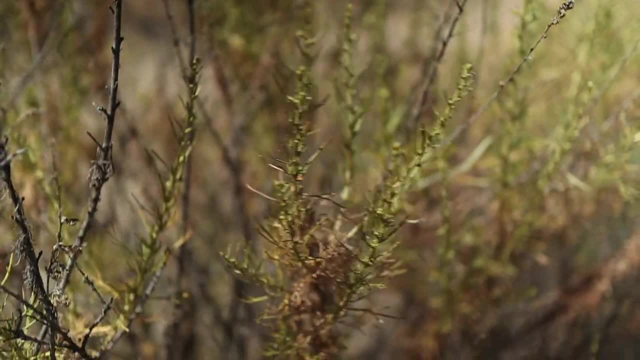 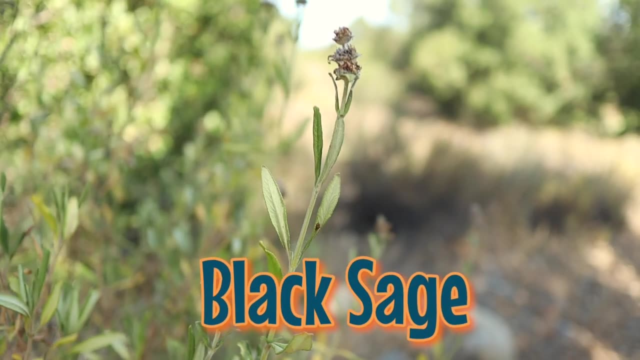 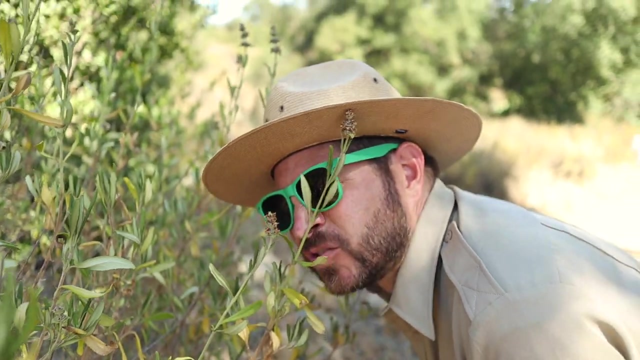 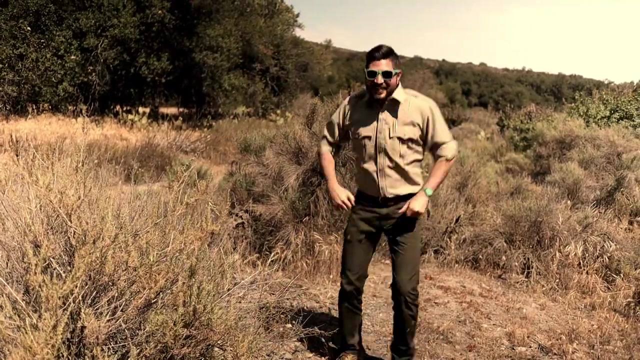 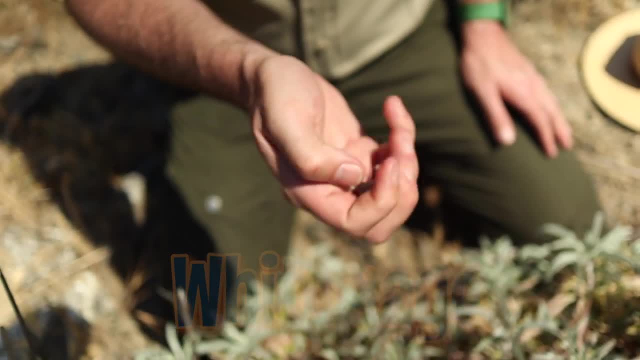 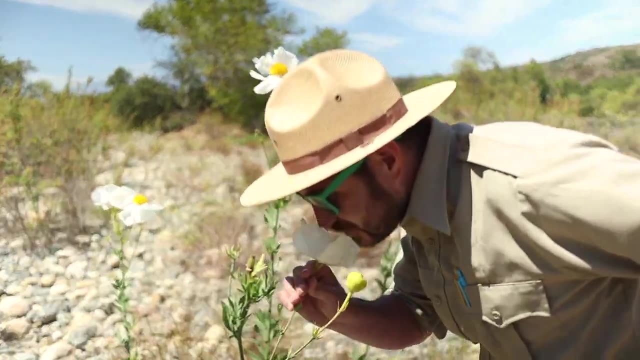 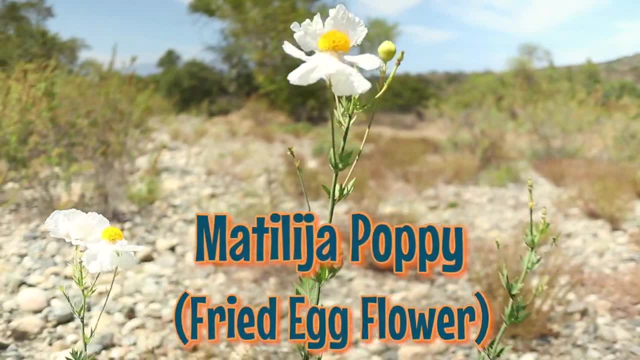 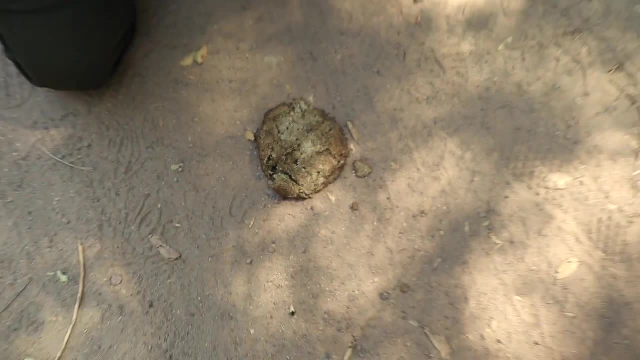 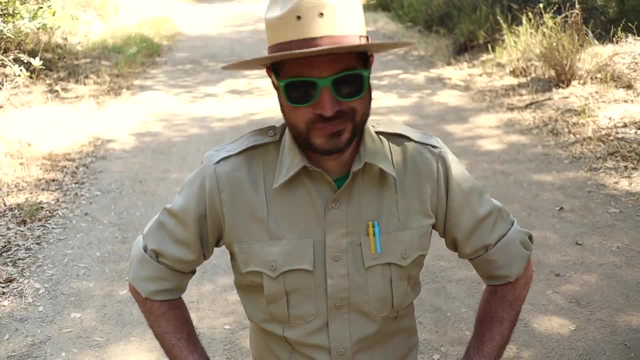 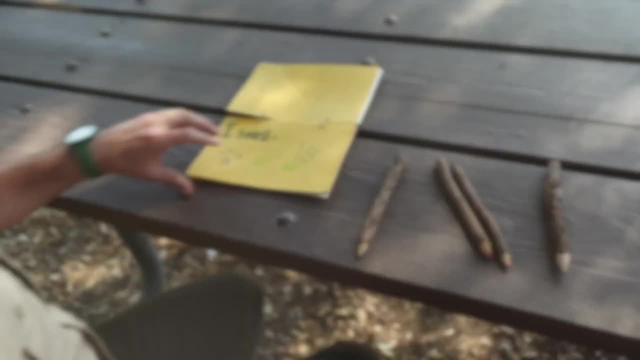 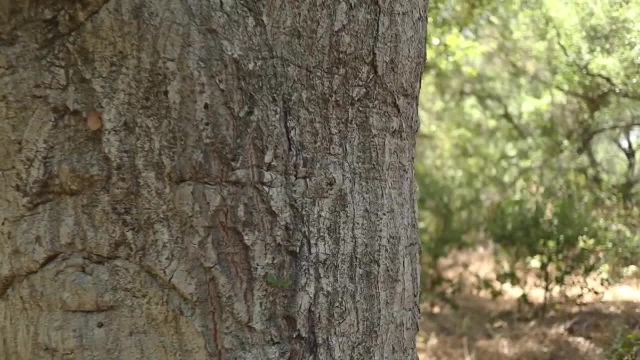 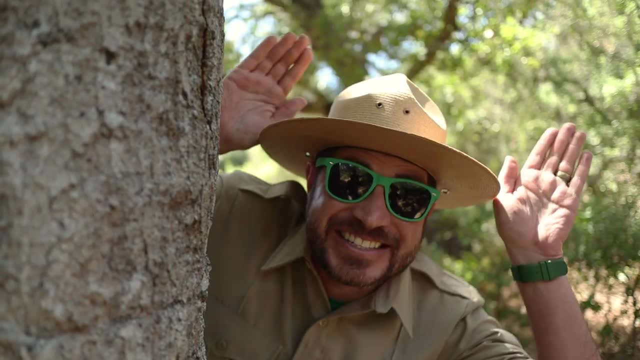 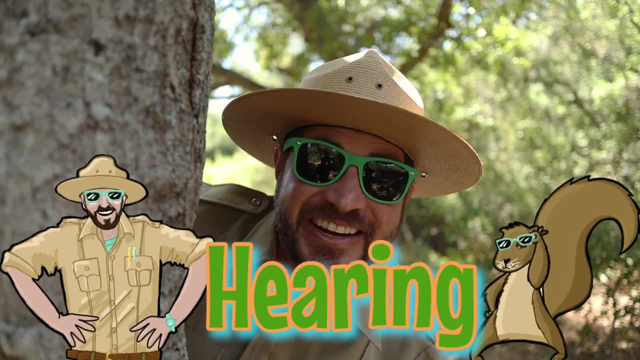 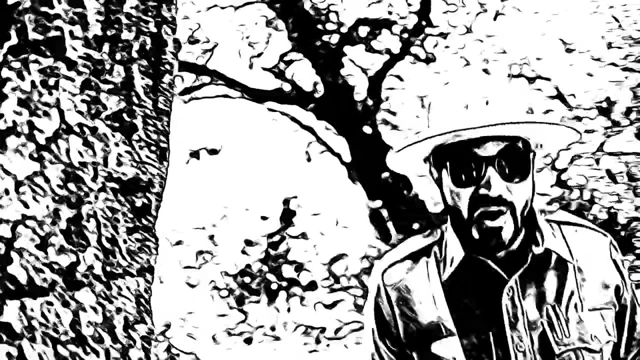 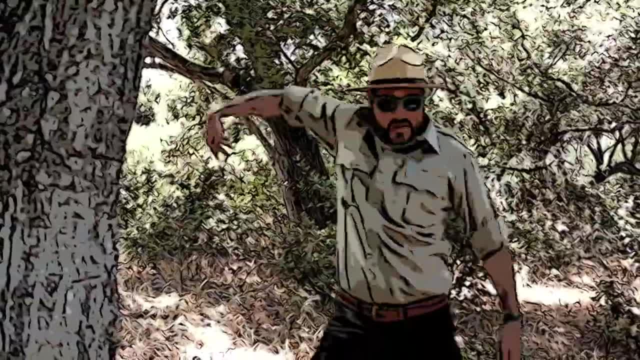 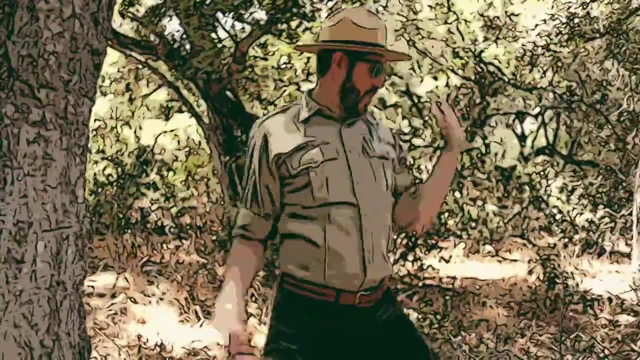 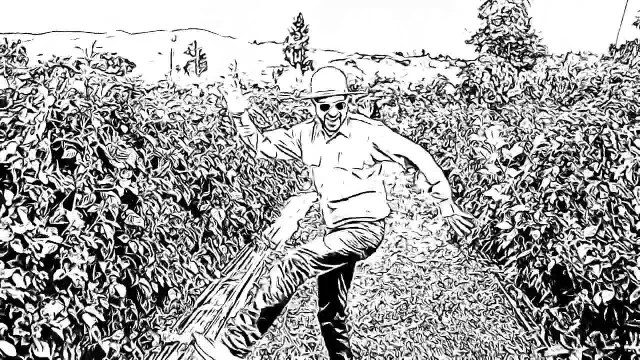 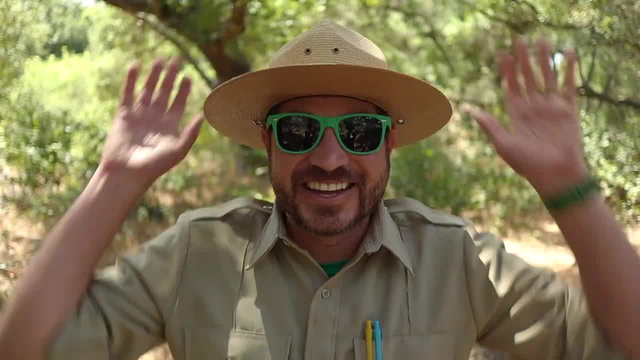 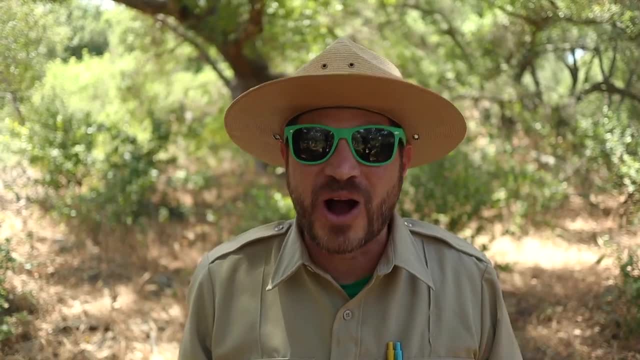 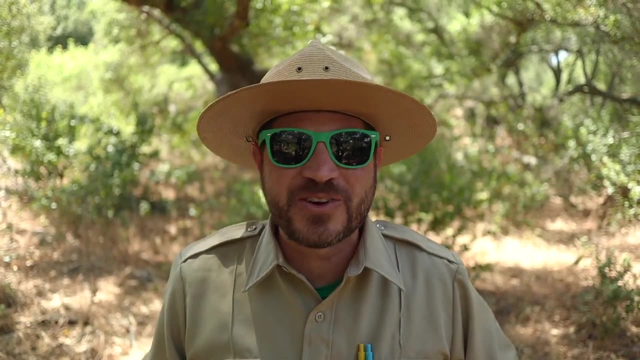 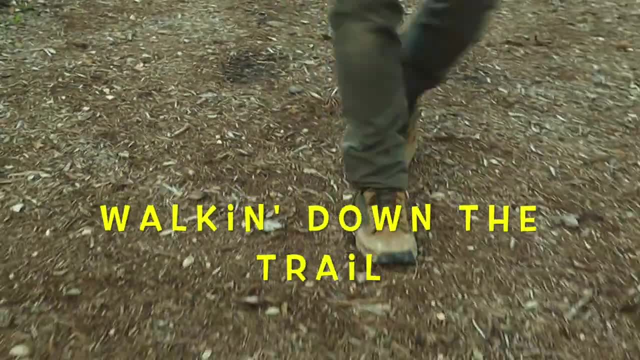 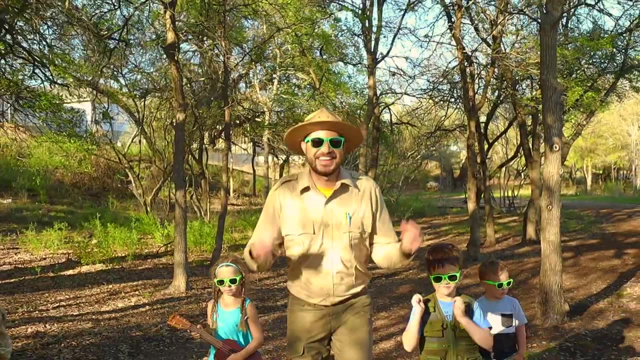 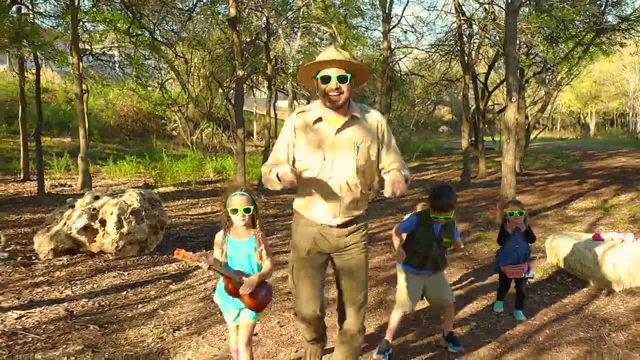 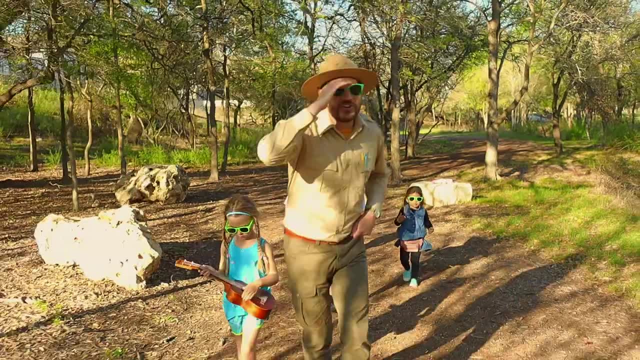 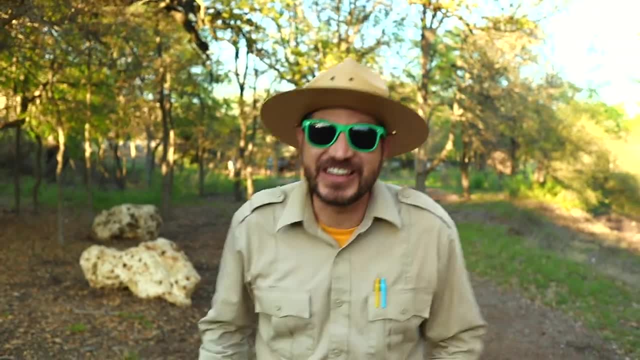 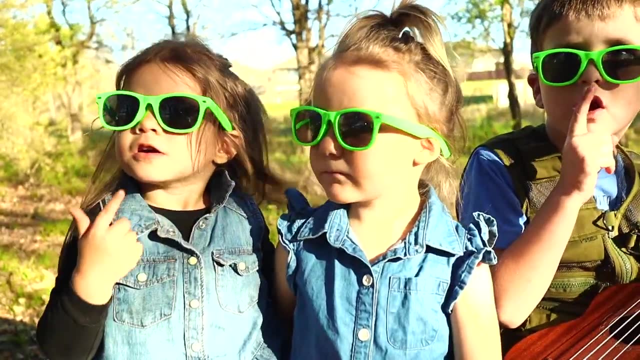 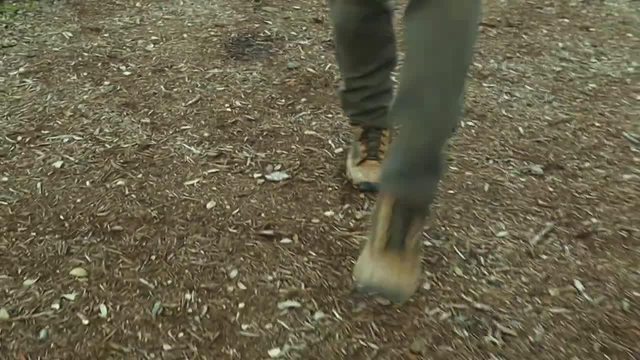 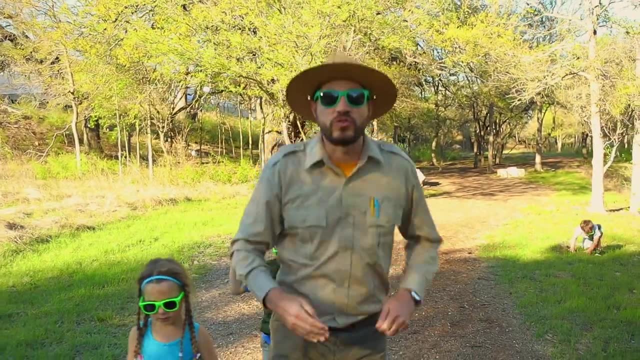 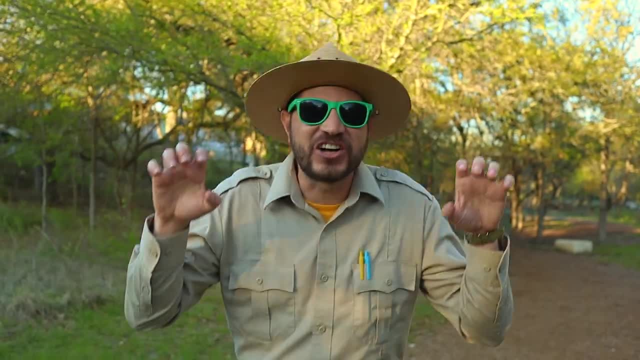 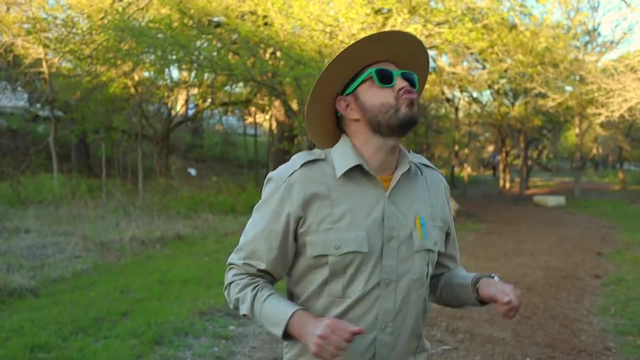 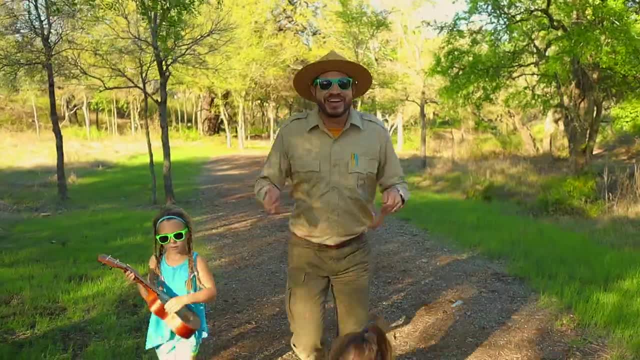 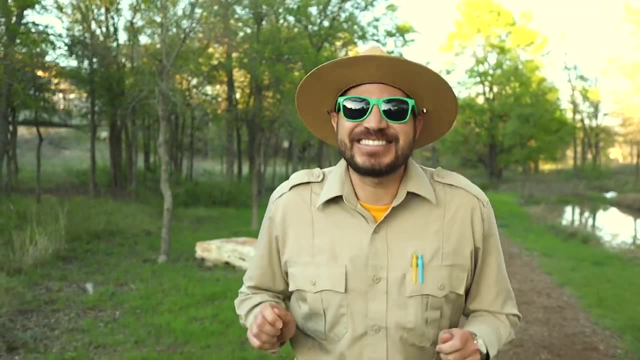 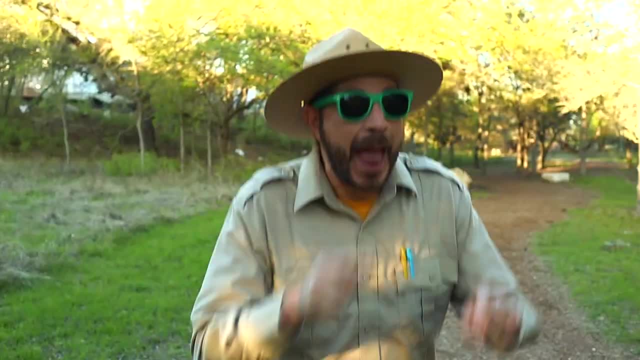 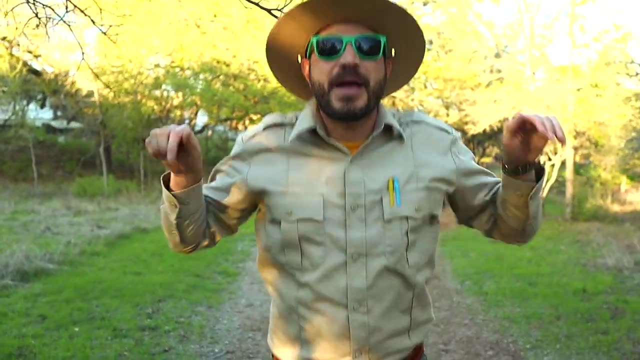 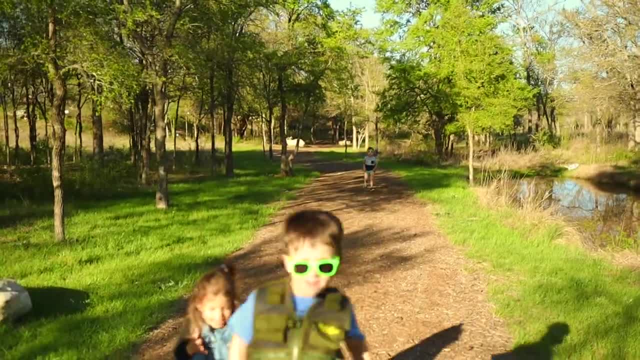 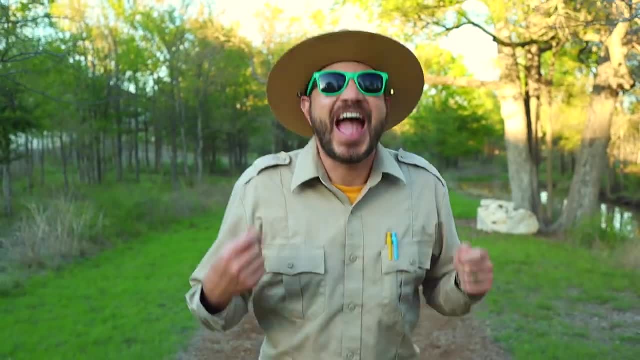 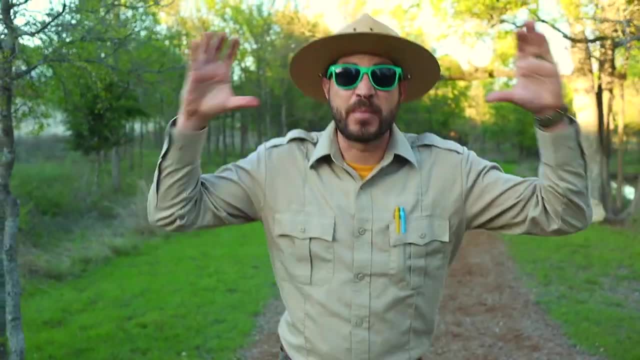 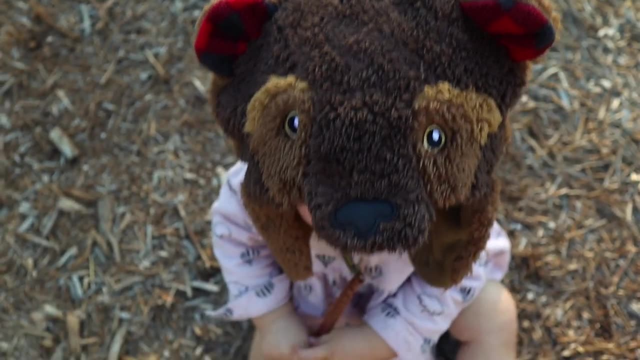 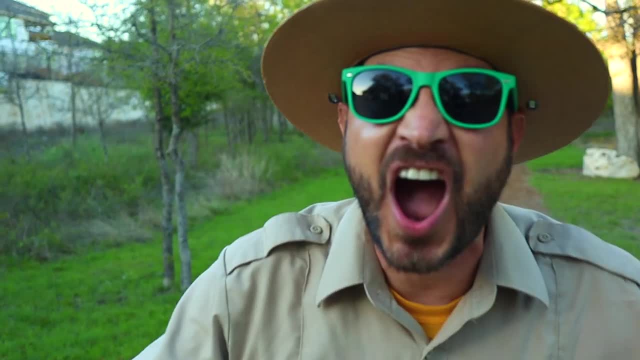 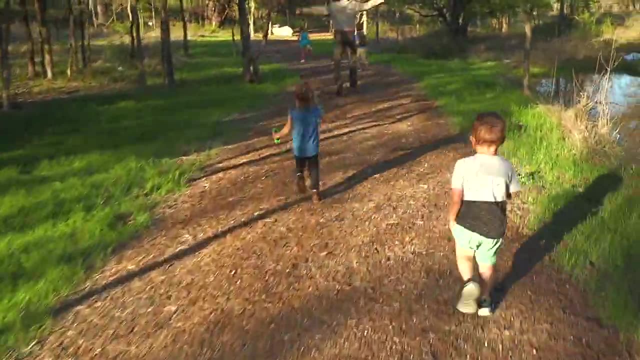 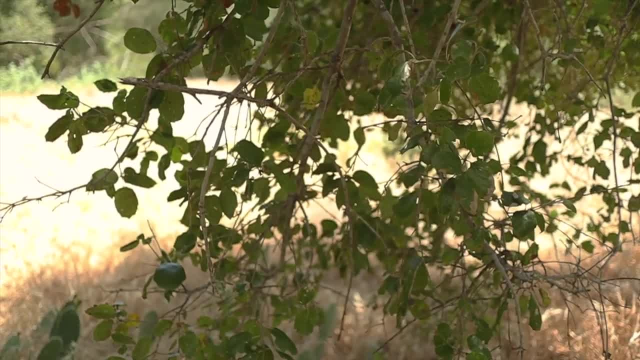 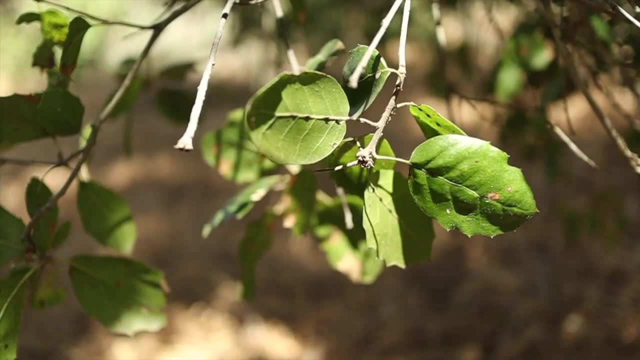 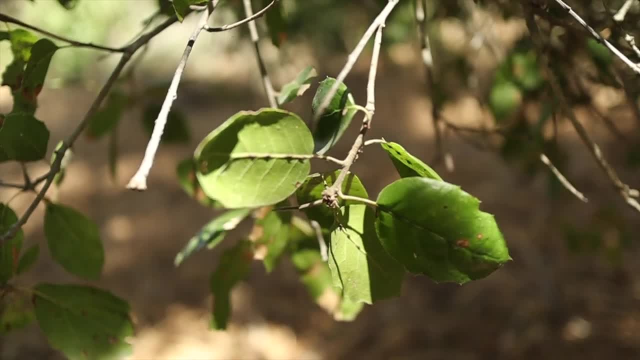 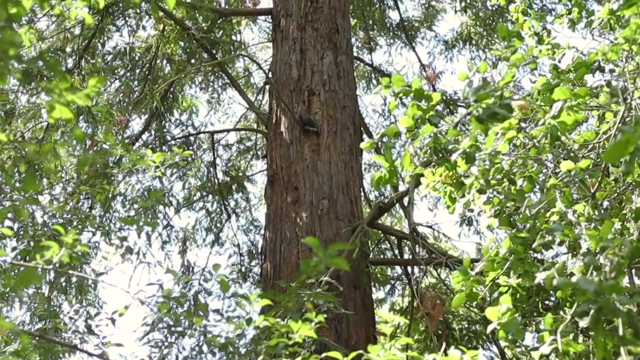 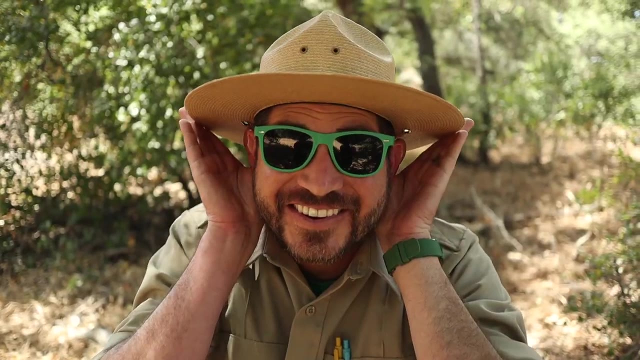 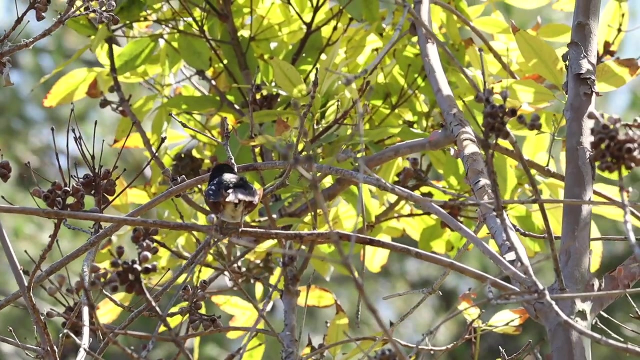 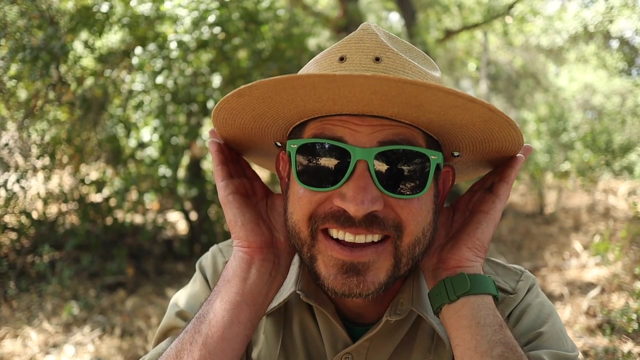 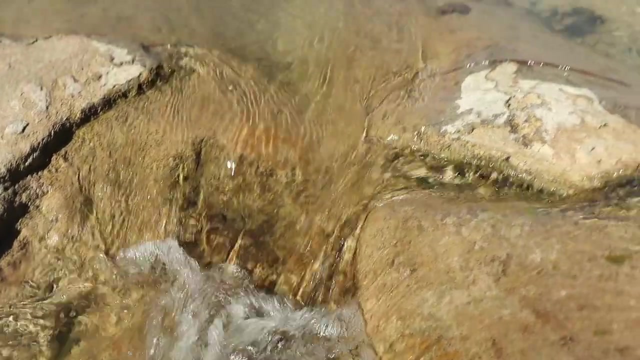 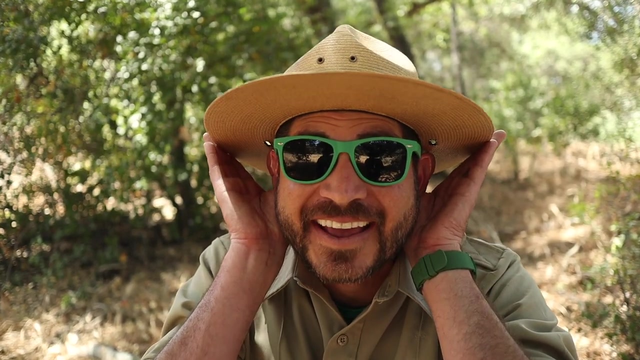 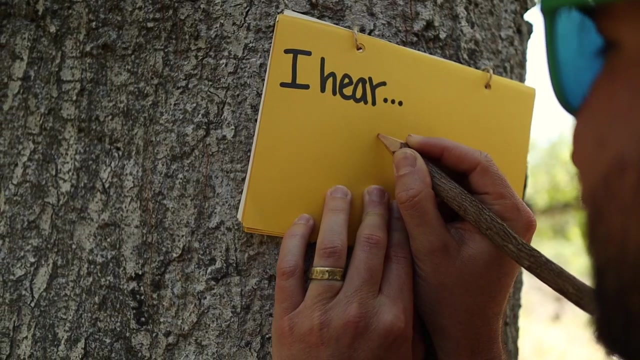 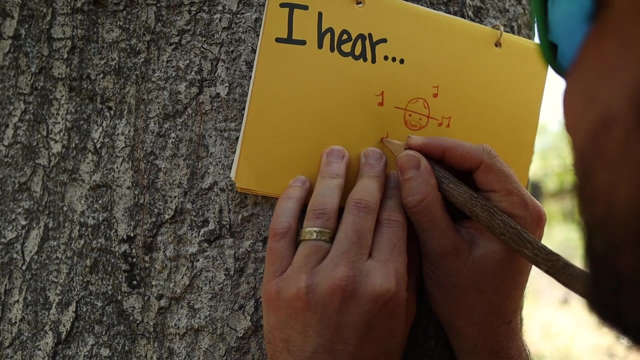 Yee-haw, Yee-haw, Yee-haw, Yee-haw, Yee-haw, Yee-haw, Yee-haw. Do you hear those woodpeckers? Do you hear those birds? It sounds like there's a creek nearby. 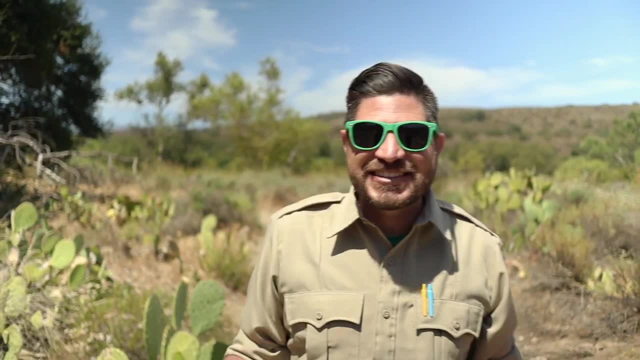 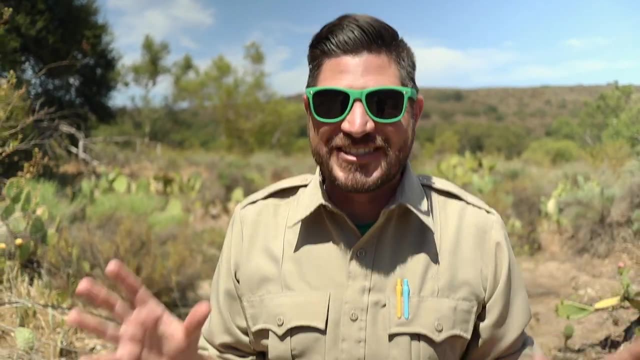 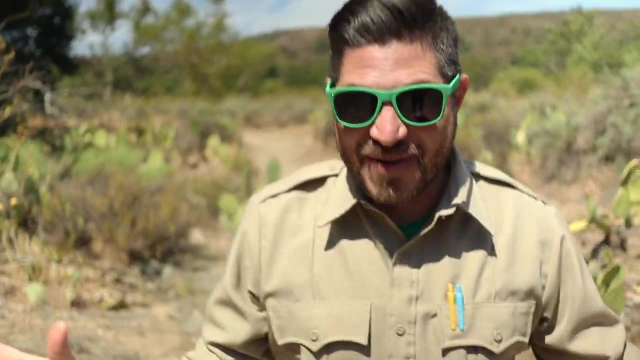 Next up on our Observation Skills, Nature Hike is our Sense of Touch. Our skin has receptors in them that can tell us a lot about the things that we touch, Or that touch us. Oh, Try to keep up, Junior Rangers. While we have the sense of touch all over our bodies, one of the most sensitive areas- 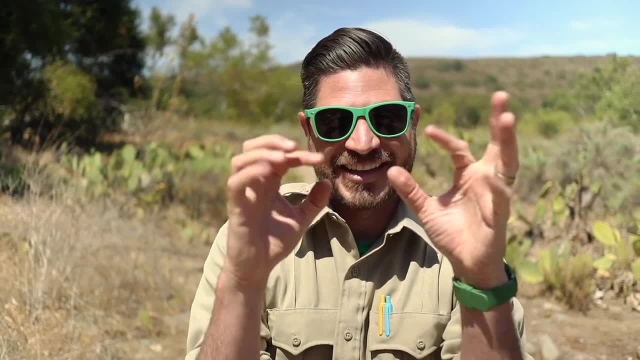 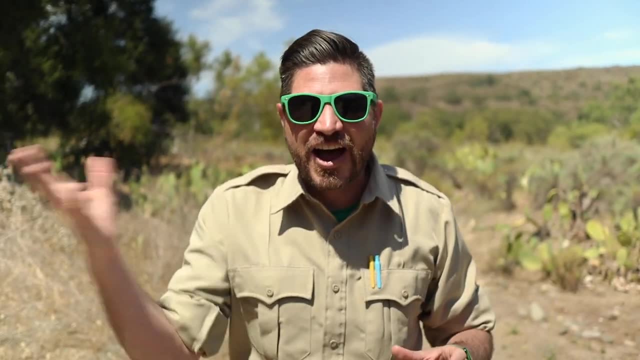 are- you guessed it- our raccoon hands. With these little bad boys, we can tell a lot about the natural world around us. They can tell us if a rock is hot or cold, if grass is wet or dry or if a leaf is smooth. 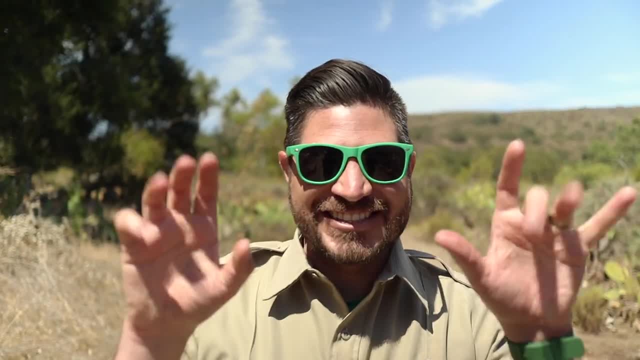 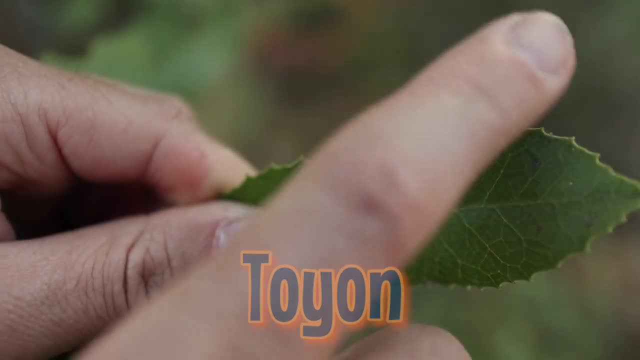 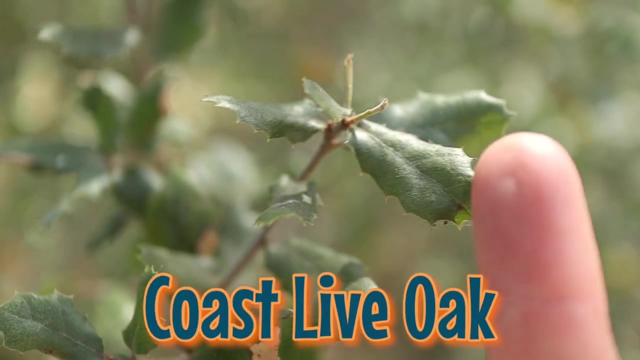 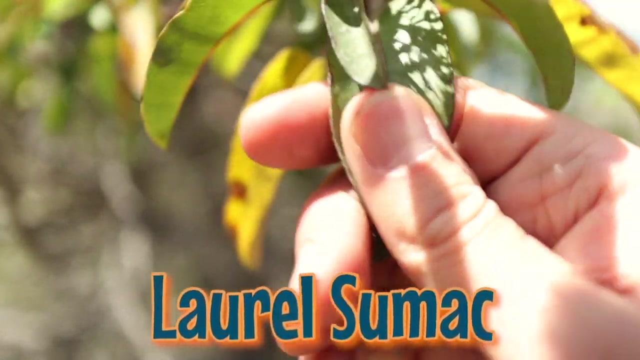 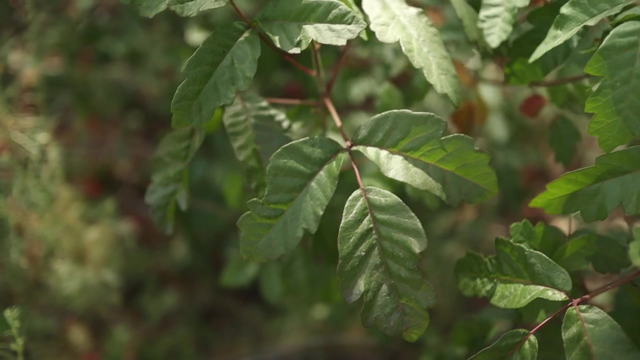 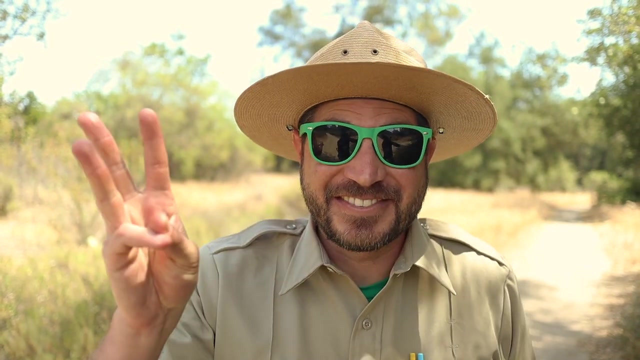 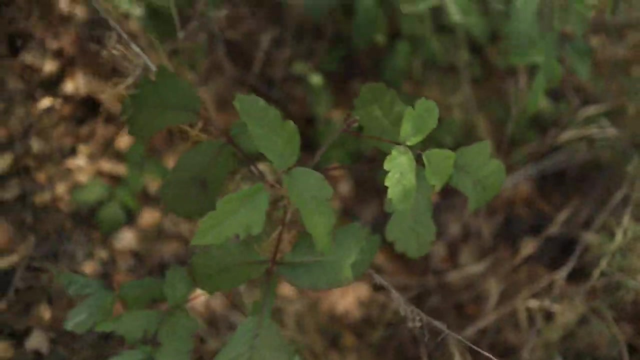 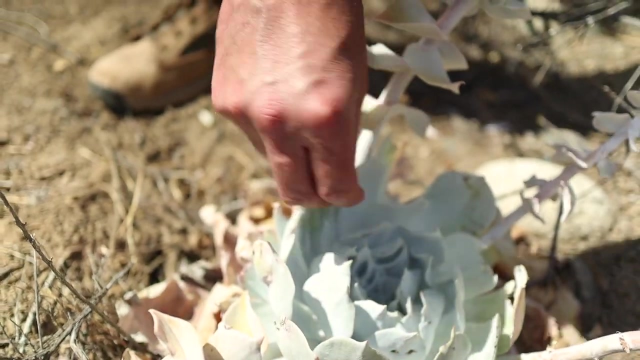 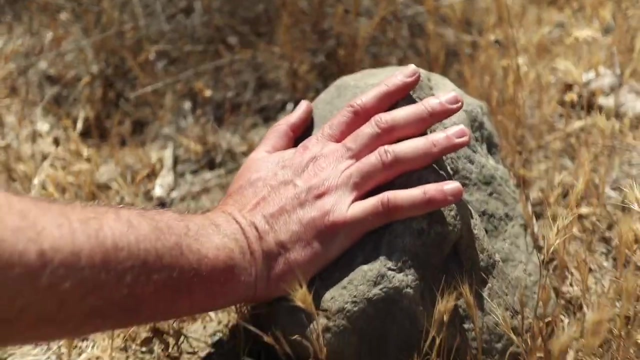 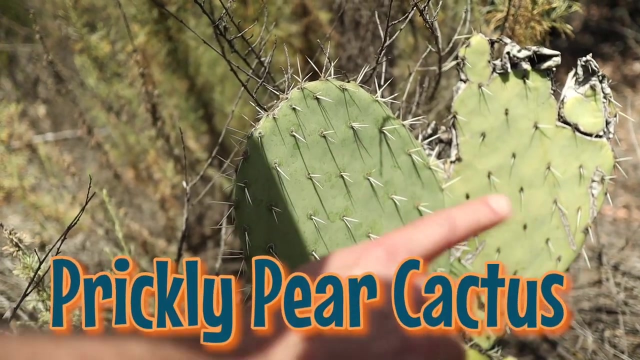 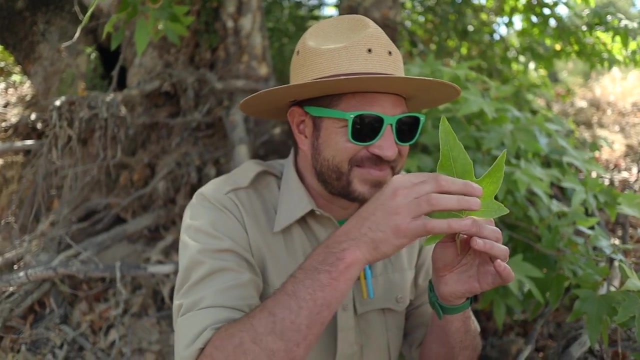 or rough. Let's check out some things with our raccoon hands now. Don't use your raccoon hands on that one. It's poison oak. Remember leaves of three. let it be Hot, hot, hot, hot, hot. 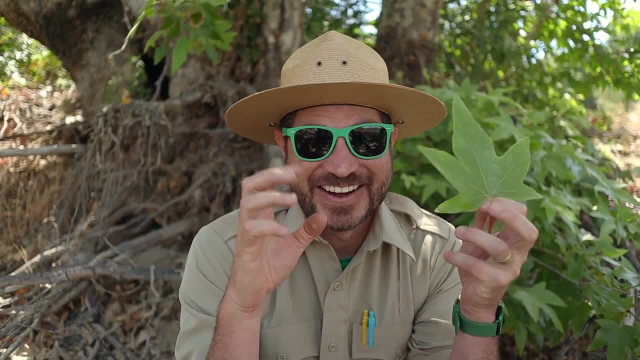 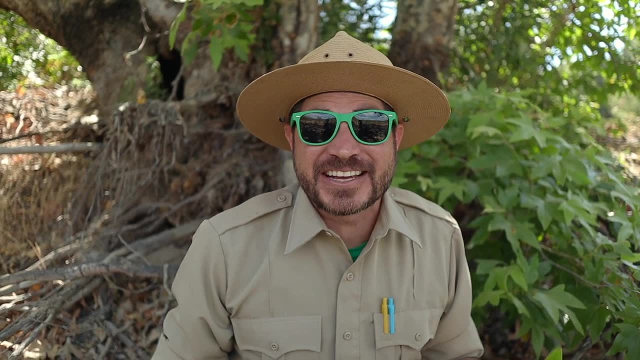 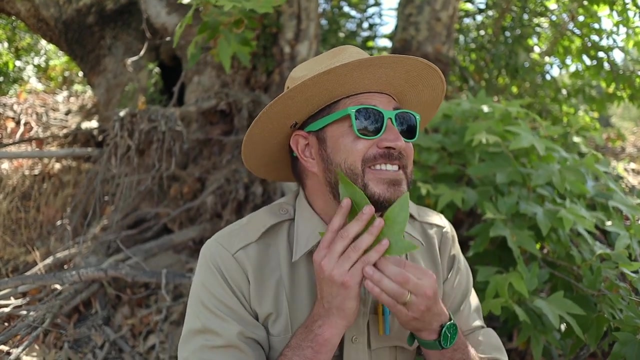 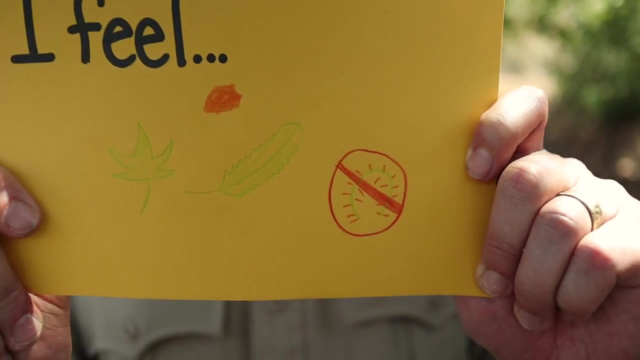 Sycamore leaves are really fun to use your raccoon hands on. They're fuzzy, making them soft to the touch. This special adaptation helps the sycamore tree stay nice and cool and hold on to its skin. Ah, so soft. 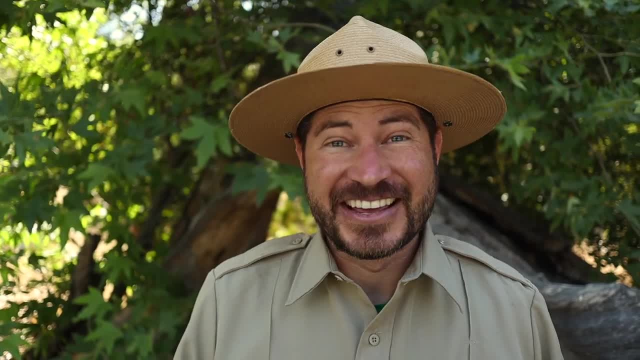 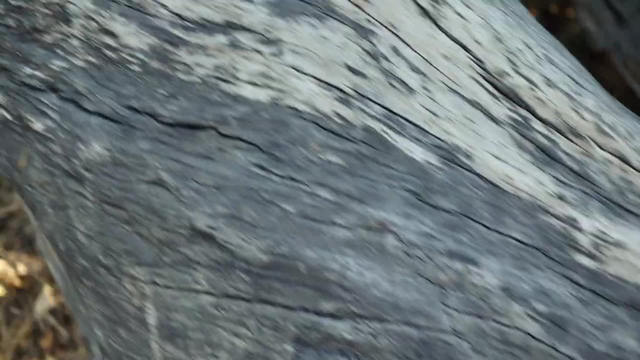 Are you ready for your Ranger's Act? fun fact? Yeah Well, here it is. The sycamore tree has one of the largest leaves in North America. It's nicknamed the ghost tree because of its white bark and soft leaves. Its shade is named Whitebark and it has a spooky shape. 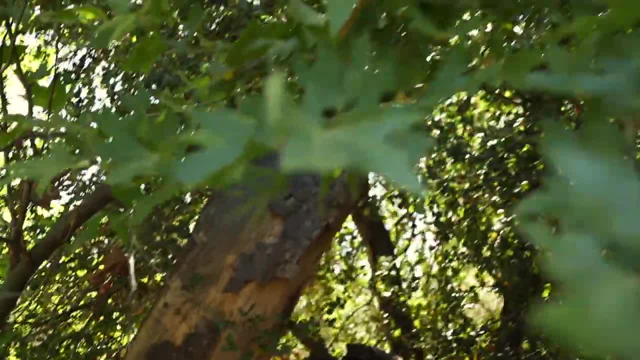 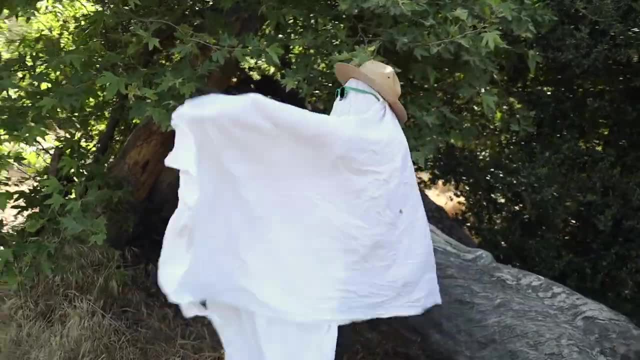 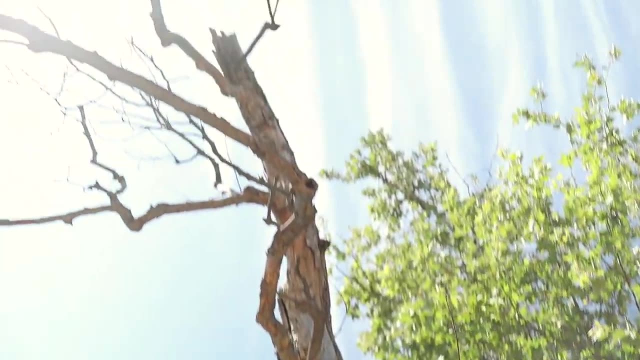 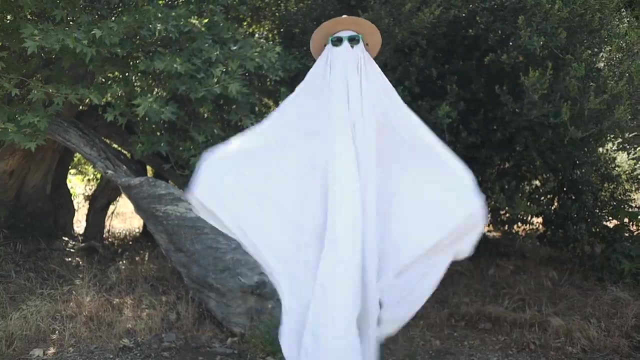 Woooooooohooooooooooo, Whooooooo, Whooo, Belaaaauuuugh, Whoooooooooooooo Whooo, Whoooooooooo, Whooooo, Whooooo, Whoooooooooo, Whooooooooo, Whooooo. 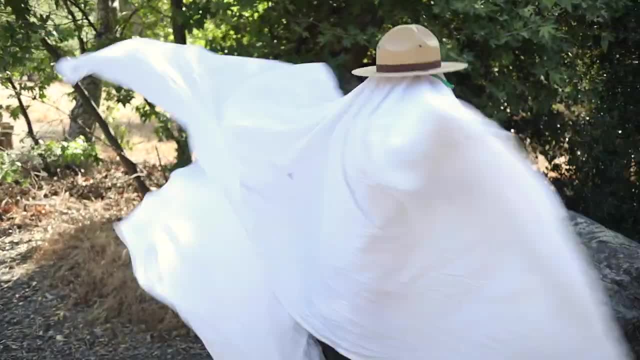 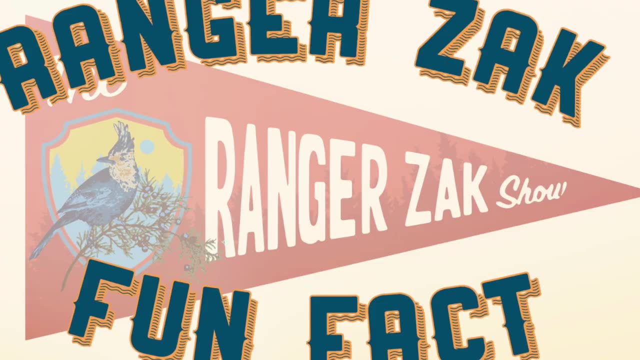 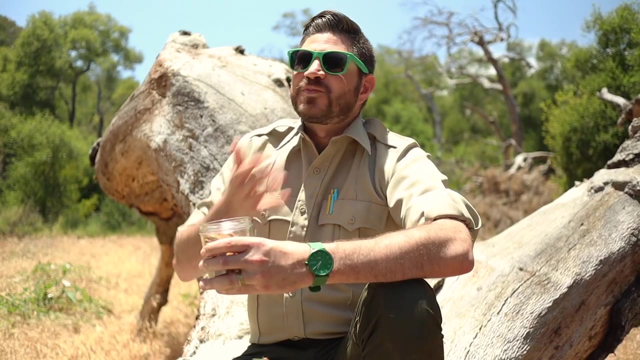 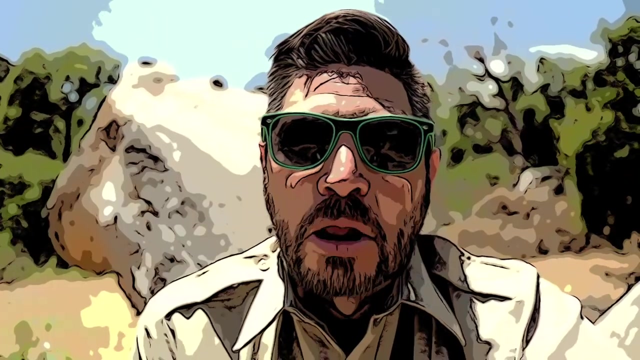 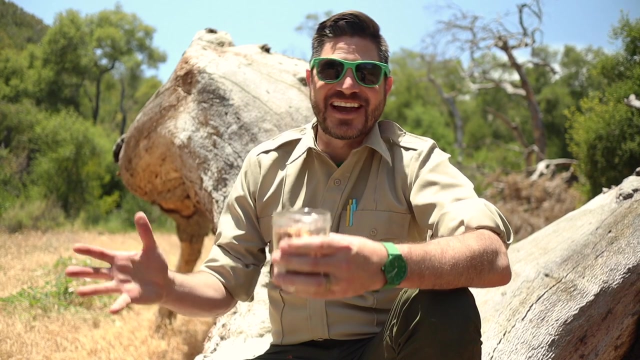 Whooooo. Well, I don't know about you, Junior Rangers, but I've worked out quite the appetite. Mmm, this trail mix is good And now we're using our lizard tongues And it's the last of our five major senses, our sense of taste. 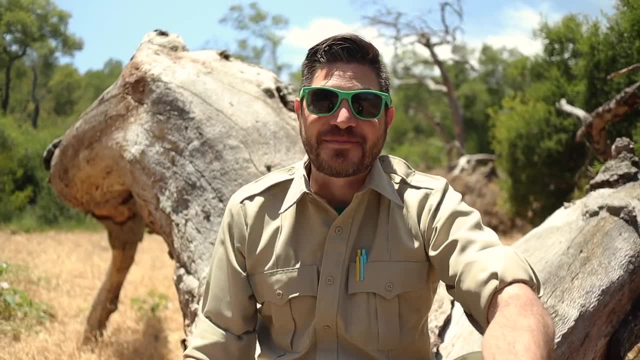 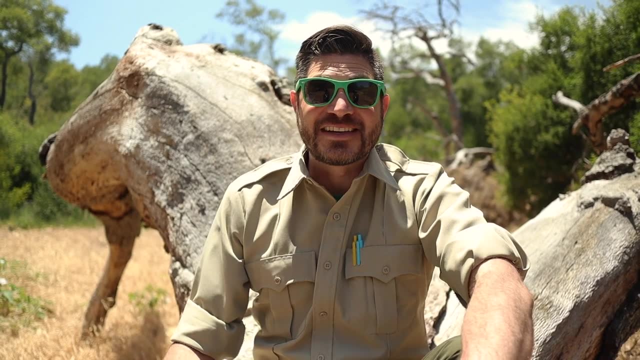 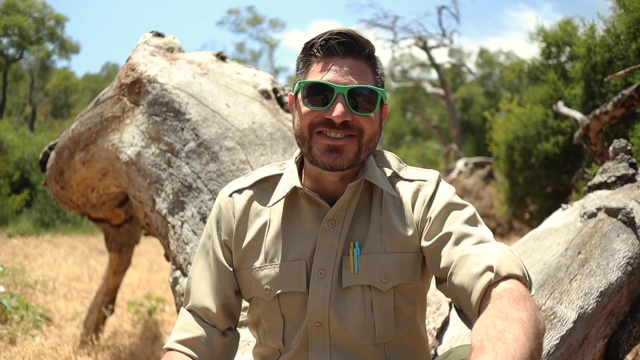 Did you know that your tongue is covered in tiny receptors that help you taste? They're your taste buds. Your taste buds tell you if something tastes sweet, sour, salty or bitter, And while there are things out in nature that you can eat, never taste anything that you. 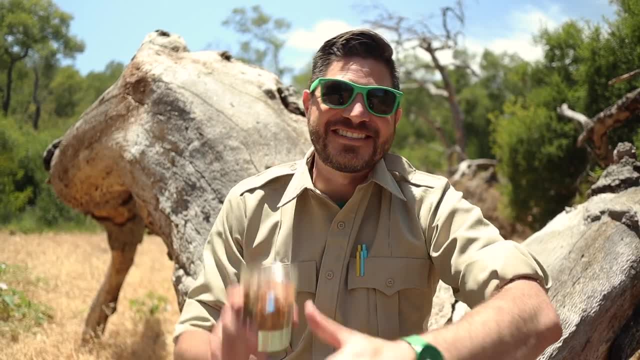 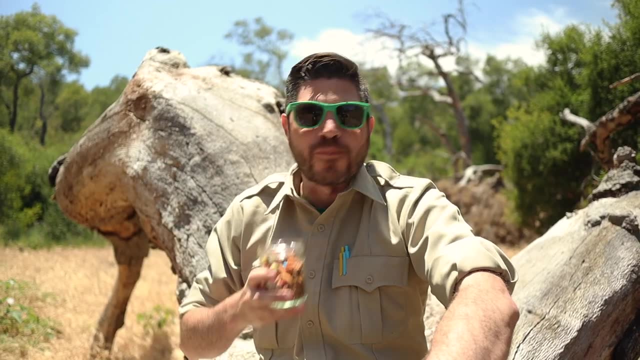 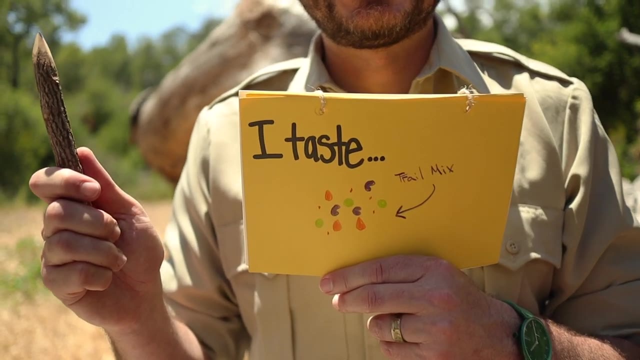 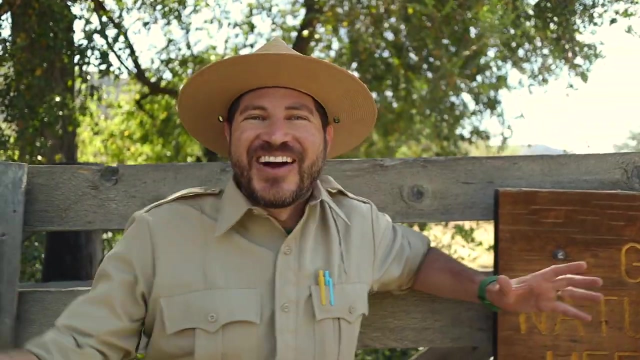 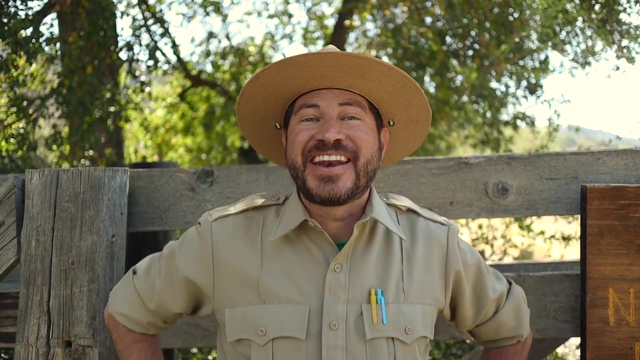 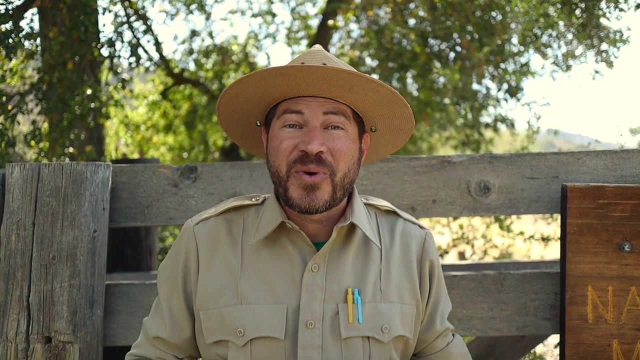 find on the trail without the help of an expert Stick to trail mix. Well, Junior Rangers, thanks for coming on the observation hike with me. As you can see, there are lots of ways to explore the natural world around you. So the next time you're out on a hike, don't just stop to smell the roses, feel the wet. 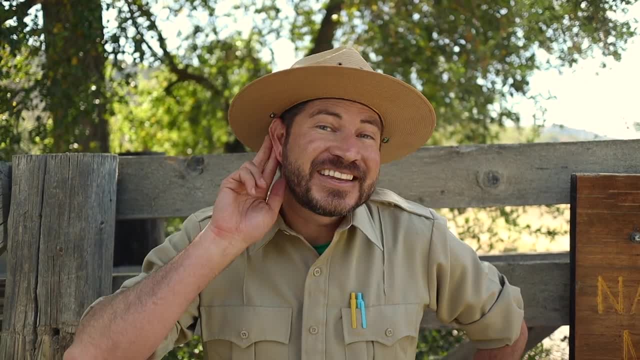 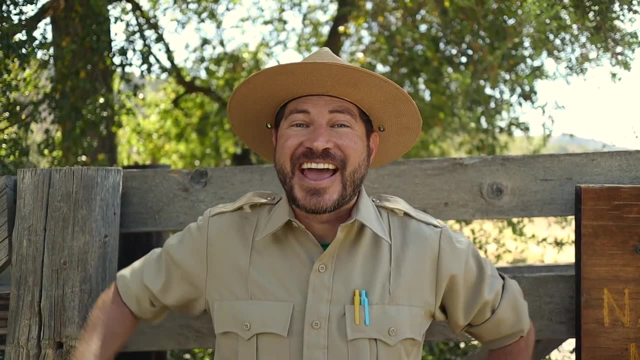 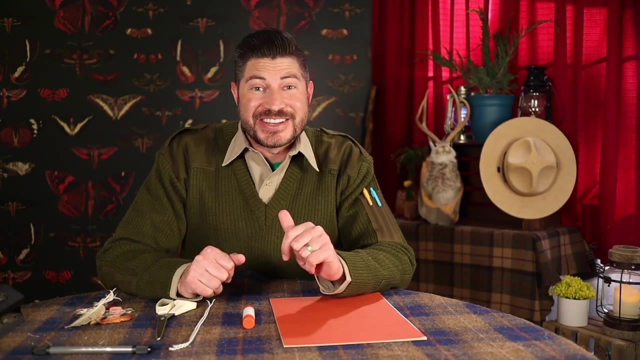 sand below your feet, watch a caterpillar roam, listen to a babbling brook and enjoy the fresh flavors created by nature. Let's head back to the ranger station and wrap things up. Hey Junior Rangers, welcome back to the ranger station. 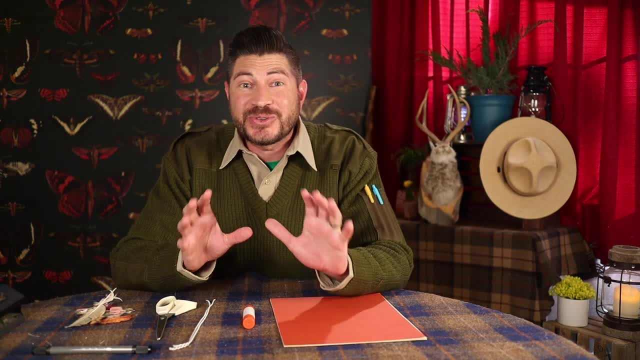 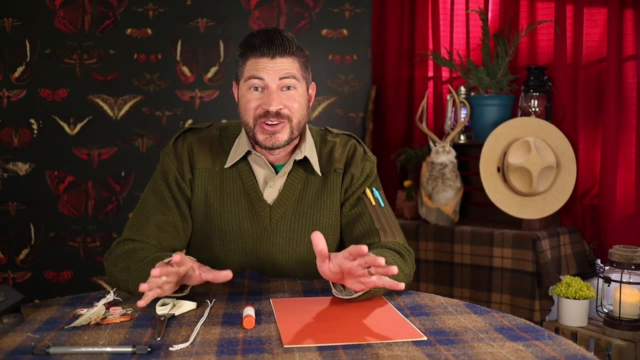 We learned today that there are lots of ways to explore the natural world around you and a great way to document your experience. The best way to document all your observations is in a nature observation journal, And today I'm going to teach you how to make your very own. 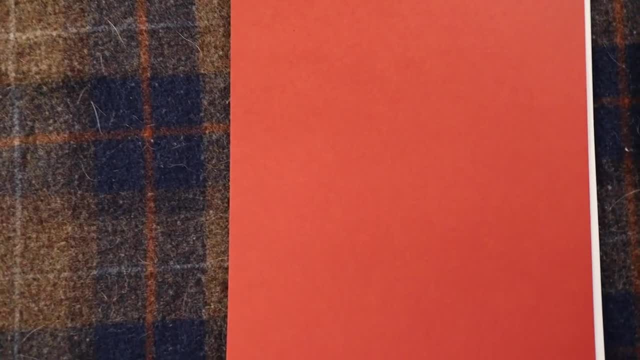 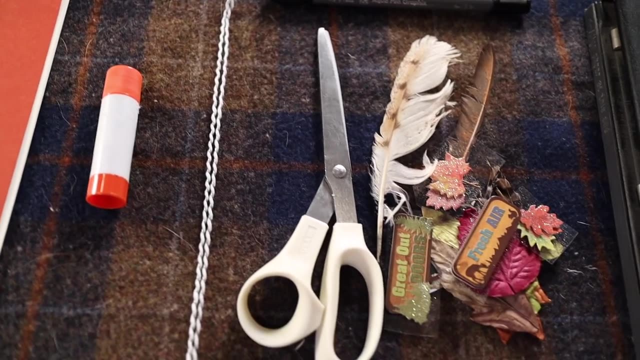 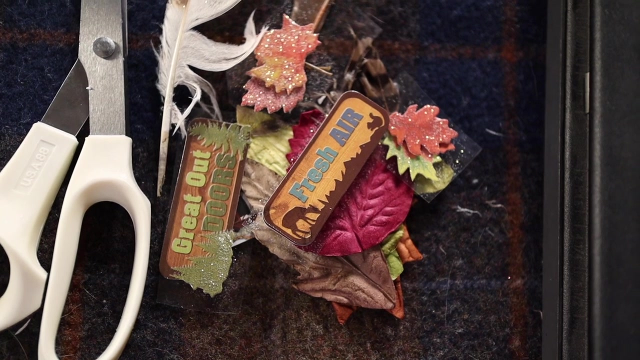 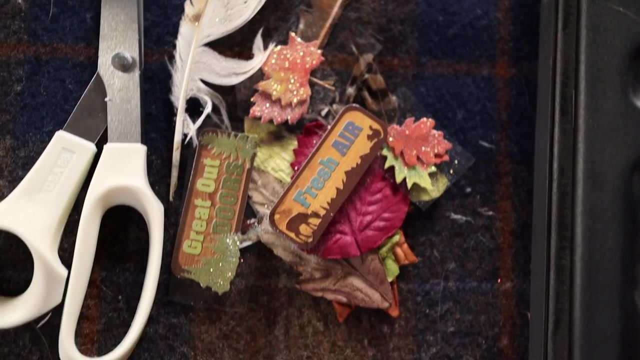 For this project you need some brightly colored construction paper, a glue stick, some twine, a pair of scissors, a marker, some decorations. these can be feathers, twigs, leaves, stickers- anything you want to use to make your nature observation journal special to you- and a 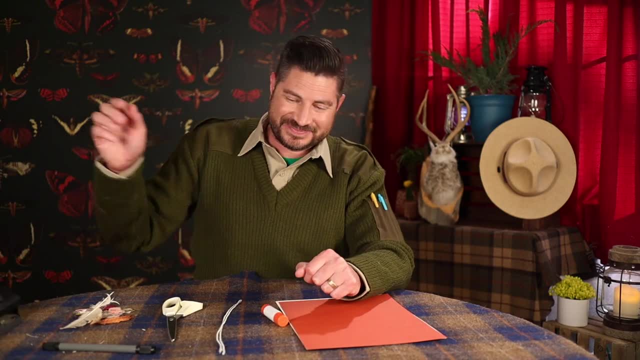 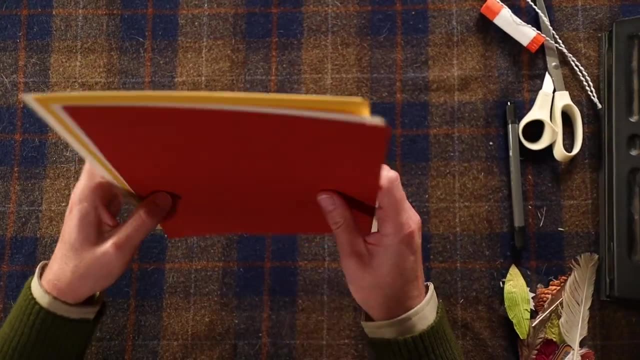 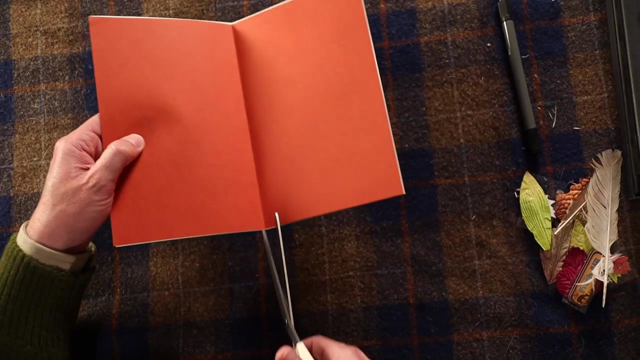 hole puncher. Punch, Punch, Punch. Let's get started. Let's start by taking a few pages of construction paper and folding them in half. Next, take your scissors and cut along the crease. This creates the pages of your observation journal. 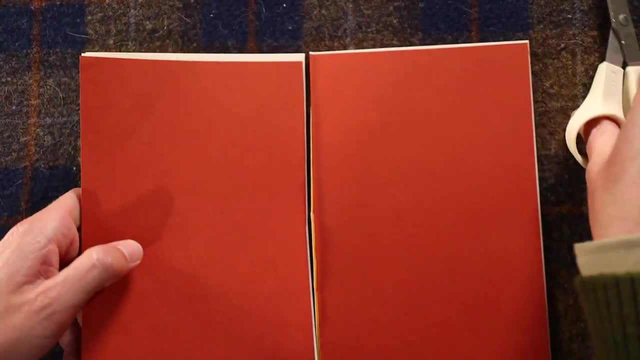 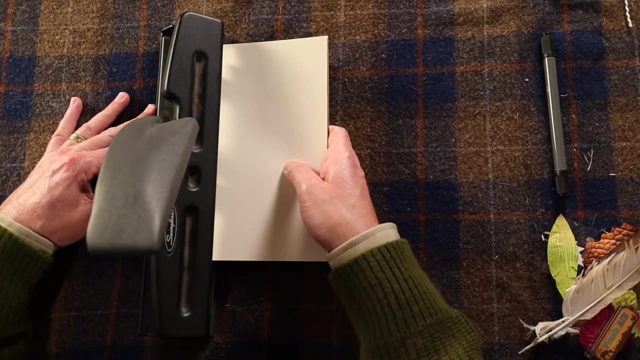 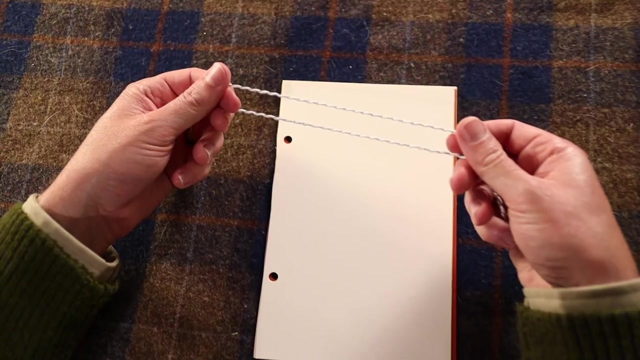 This creates the pages of your observation journal. This creates the pages of your observation journal. Take a hole puncher and punch two holes through the pages. Take some twine and tie them loosely through the holes. This will keep all your pages together.